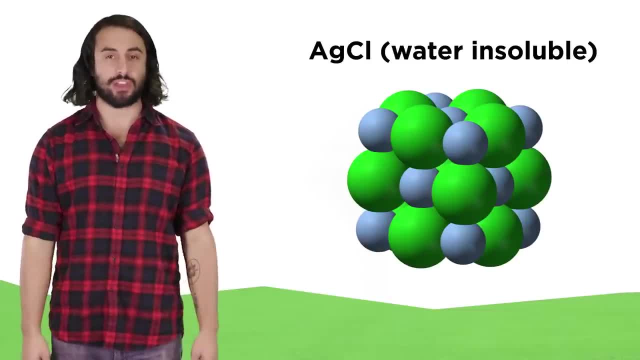 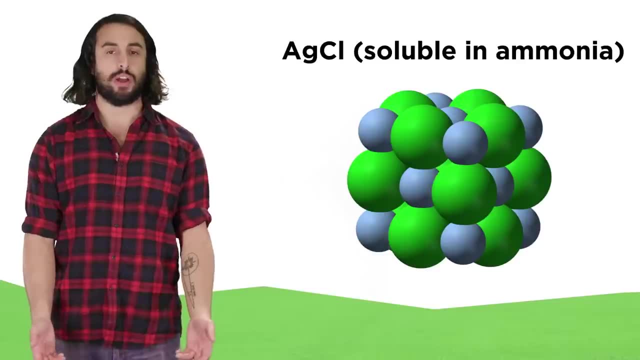 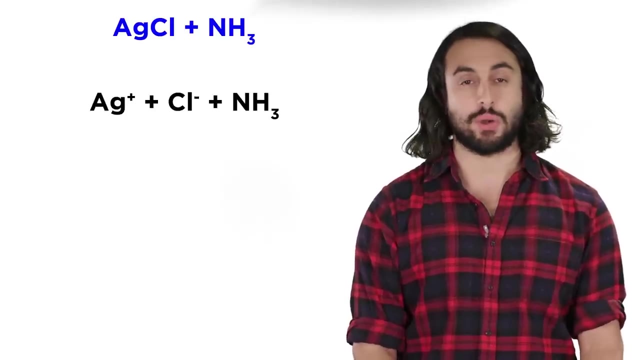 in the solid phase is greater than the energy of solvation that will result if the ions break apart. however, silver chloride is somewhat soluble in ammonia because these substances can form a complex ion in ammonia. silver chloride will dissociate and two ammonia molecules can coordinate. 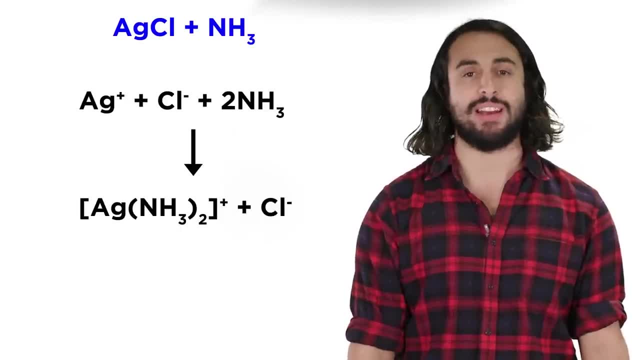 to a silver ion to form this complex ion and the chloride ion. because the main chemistry that is occurring is that the silver ion and the ammonia molecules form the complex ion. we can cancel out the chloride ions from both sides, as this will be a spectator ion. 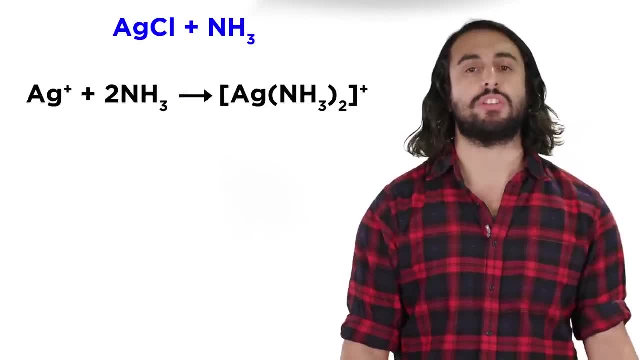 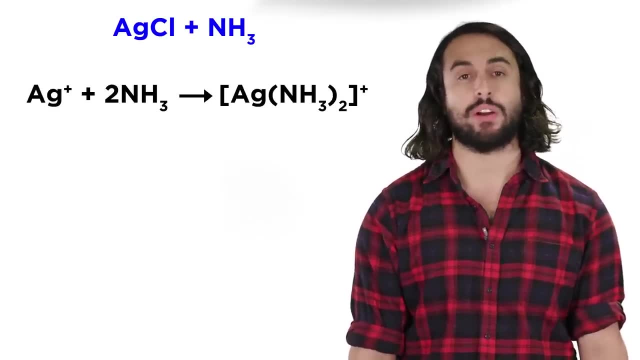 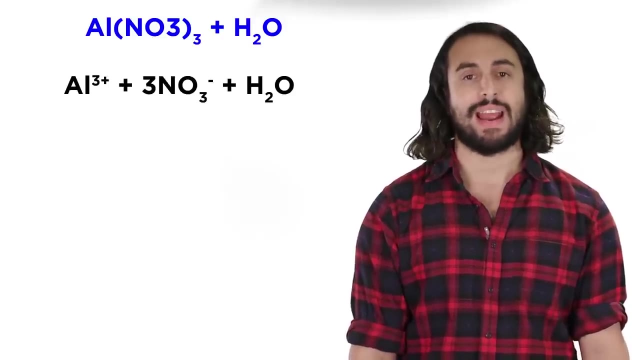 which leaves us with the following net ionic equation, which exclusively shows the formation of the ion. this doesn't happen only in ammonia. this can happen in water as well. if aluminum nitrate is dissolved in water, it will dissociate to form aluminum ions and nitrate ions, but six water molecules can. 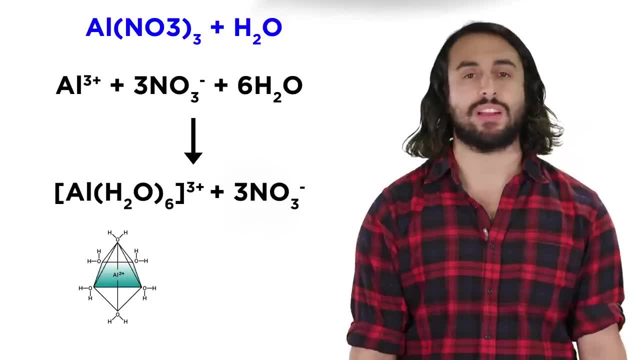 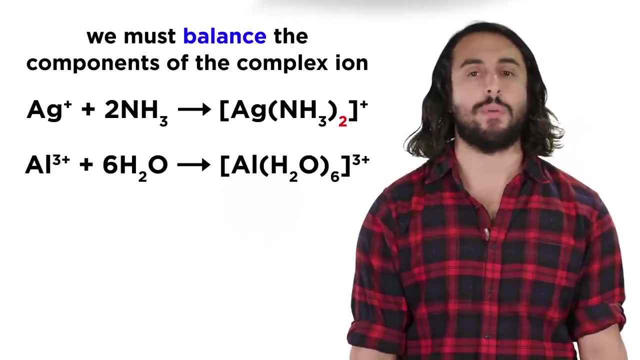 coordinate to each aluminum ion to form the following complex ion: in both of these cases we simply need to make sure each ion is balanced. if there are two ammonias in this complex ion, two ammonias must be involved on the reactant side for this one. if six water. 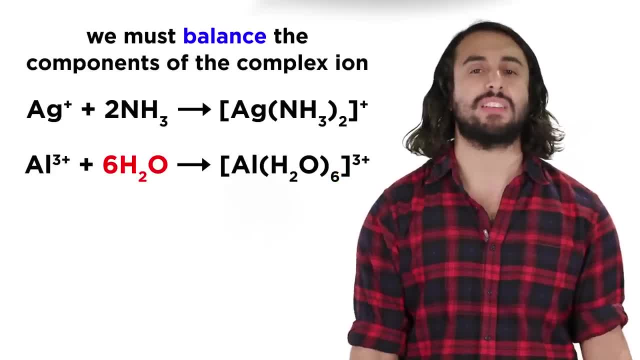 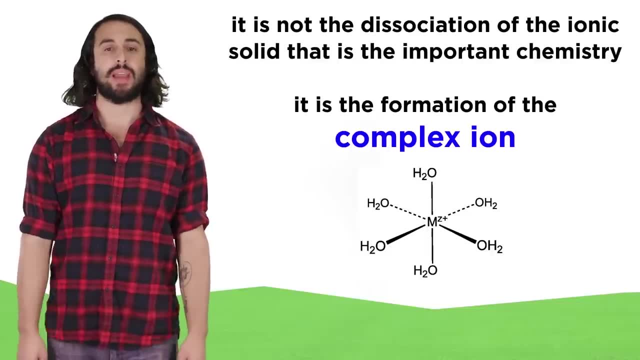 molecules are needed to form the complex ion. there must be six waters on the reactant side. once again, it is not the dissociation of the ionic compound that is the main chemistry occurring, as this is technically just a phase change. it is. 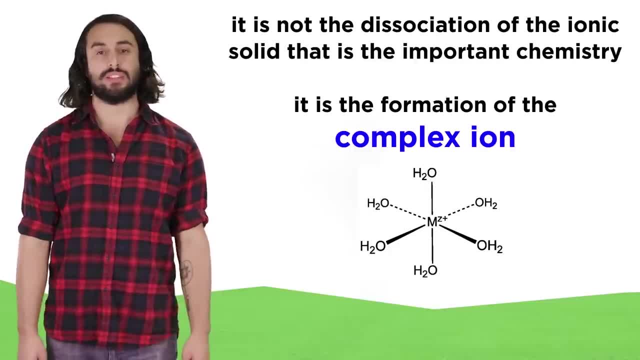 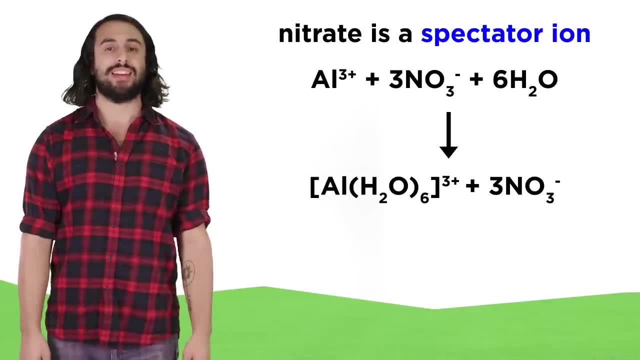 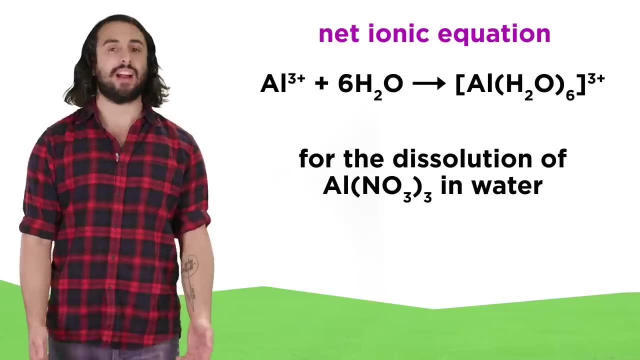 the formation of the complex ion that we really want to be discussing. for this reason, we can highlight this chemistry in the following equation and notice that nitrate is a spectator ion. this time we can cancel that out, which leaves us with the following net ionic equation: just as with other types of equations we have, 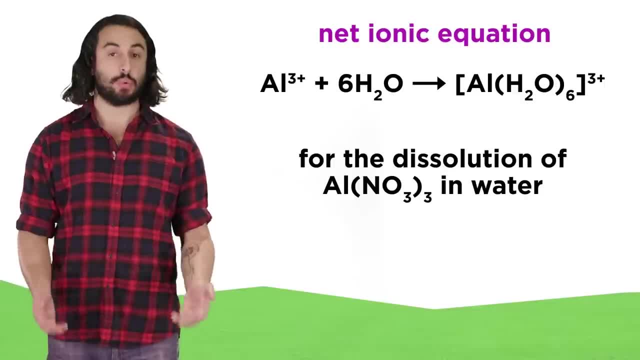 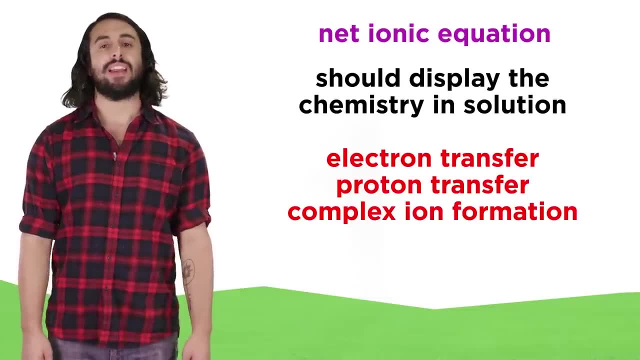 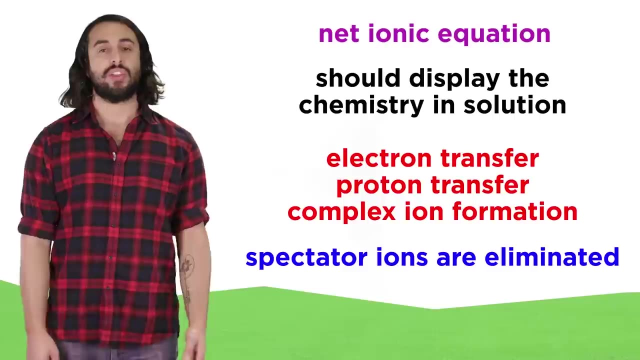 tried to balance. it is important to see what chemistry is really occurring- whether it is electron transfer, proton transfer or complex ion formation- and be able to take an overall equation and cancel out any spectator ions, to give a net ionic equation that exclusively describes the chemistry that